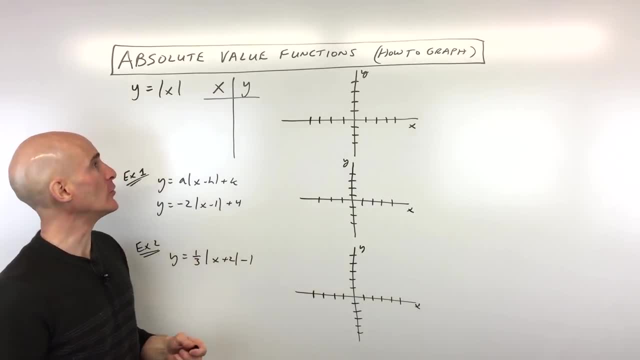 turn it into a positive number, So it's always a positive value. So let's go ahead and plot the parent function, this basic function here, by picking some negative values and some positive values. Okay, so when I put negative three in the absolute value, that's really telling. 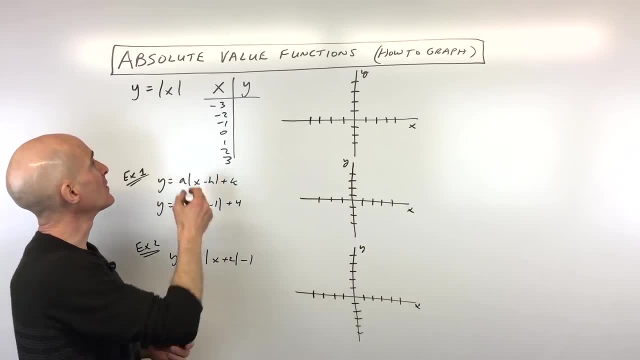 us. you know, like what's that distance from zero, Is it? you know how far is it from the, you know, from zero? Well, if you were to go on the number line, you can see here's negative three. It's actually three units from zero. Granted, it's three to the left. 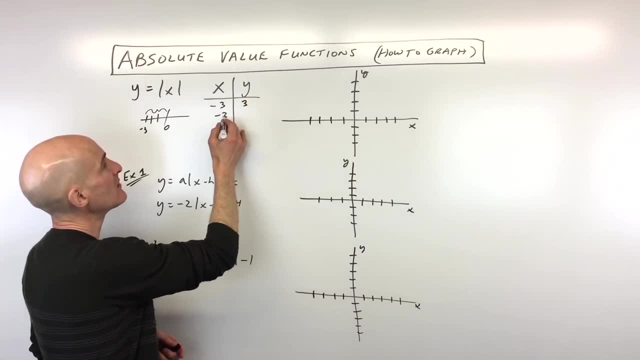 but that distance is always positive. So this is going to be three: The absolute value of negative. two: again, we make that positive. Negative one, it becomes positive one: Zero: the absolute value of zero is zero. Now, here, sometimes students make a little bit of a. 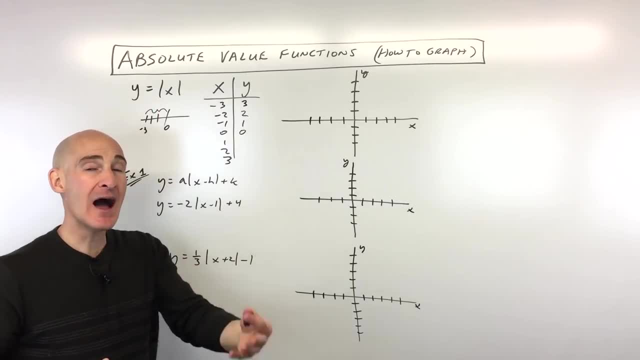 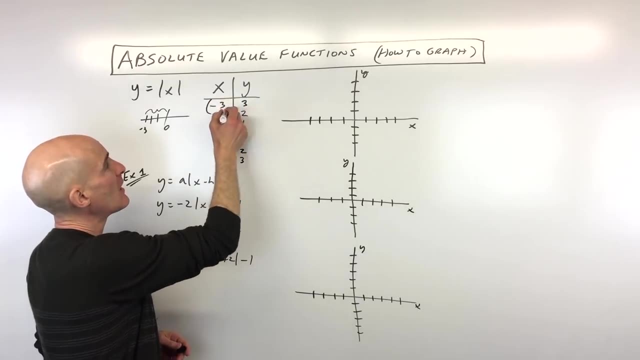 mistake. Remember: the absolute value always makes it positive. It doesn't make it. the opposite Makes it positive. So one is going to be one, two is going to be two and three is going to be three. All we have to do now is plot these coordinates from the origin. So we've. 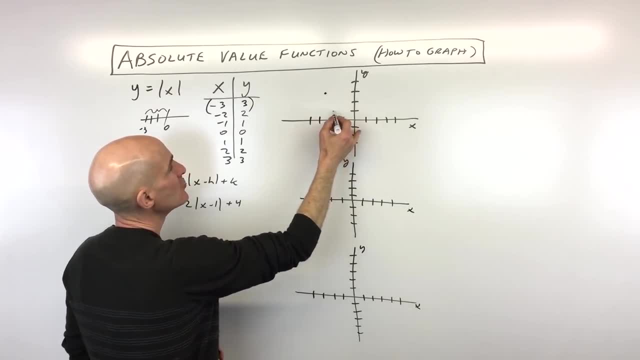 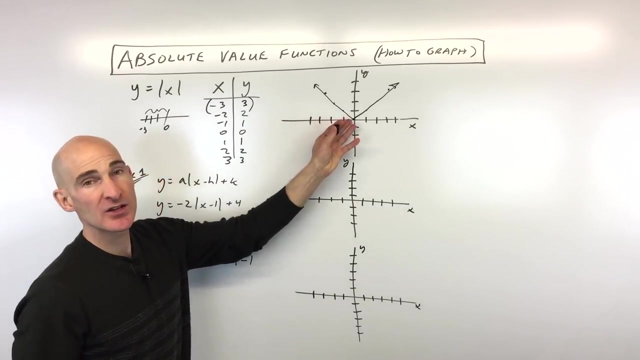 got left, three up three right, Left, two up two, left, one up one, zero zero one. one, two, two, three, three. And what you'll notice when you graph these absolute value graphs, it has that real sharp V shape, that real sharp corner to it. So that's our basic. 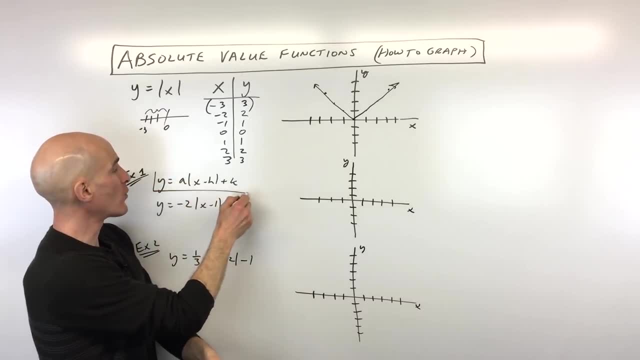 graph. But now let's say we want to do more challenging ones. Say, for example, ones that are in this form: here, Y equals a absolute value of x minus h plus k. So how does this work? Well, the h, okay. 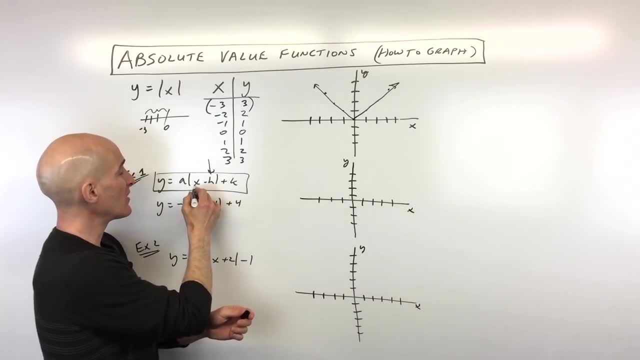 is what shifts the graph left and right. Okay, so this number that's grouped with the x, it's easy to remember. It shifts it in the x-axis direction left and right. But this one has the opposite effect on the graph. So that means if it's x minus two, it would 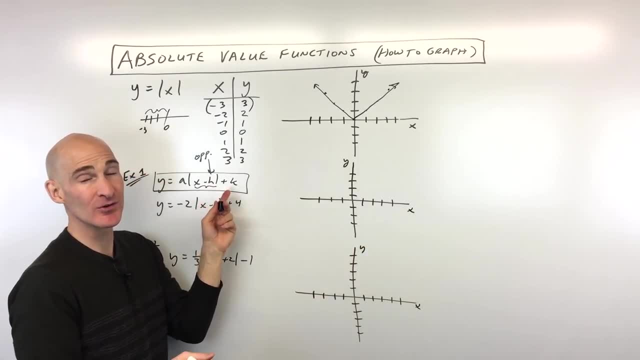 actually go positive two, so to the right. If it was x plus two, it would actually go negative two, so to the left, two. But this k value actually has the same effect on the graph, meaning if it's positive you're going to shift it up And if it's negative you're. 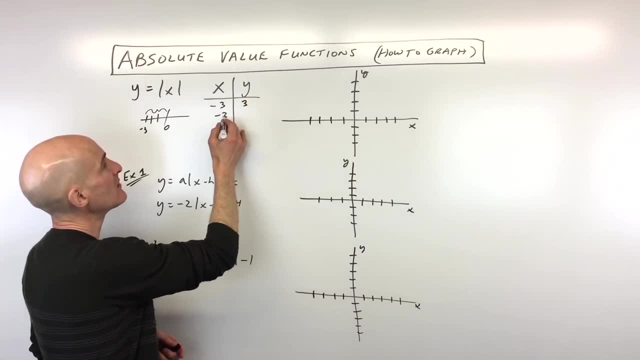 but that distance is always positive. So this is going to be three: The absolute value of negative. two: again, we make that positive. Negative one, it becomes positive one: Zero: the absolute value of zero is zero. Now, here, sometimes students make a little bit of a. 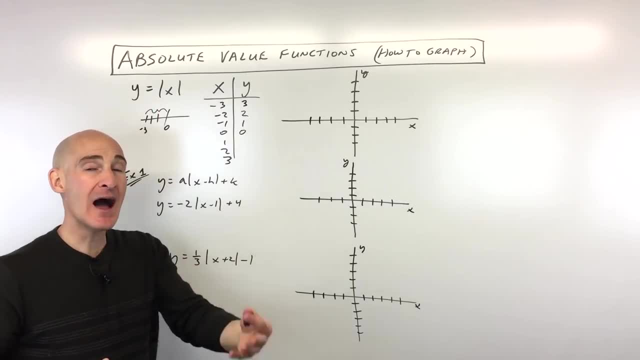 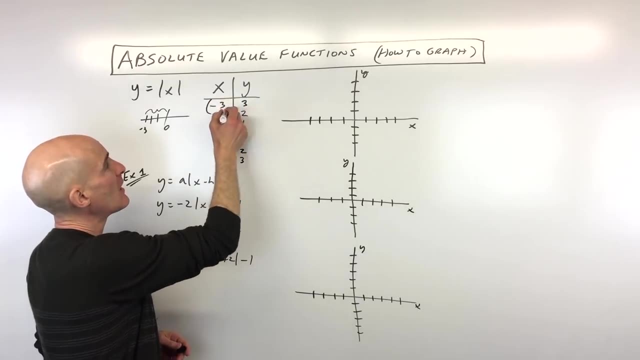 mistake. Remember: the absolute value always makes it positive. It doesn't make it. the opposite Makes it positive. So one is going to be one, two is going to be two and three is going to be three. All we have to do now is plot these coordinates from the origin. So we've. 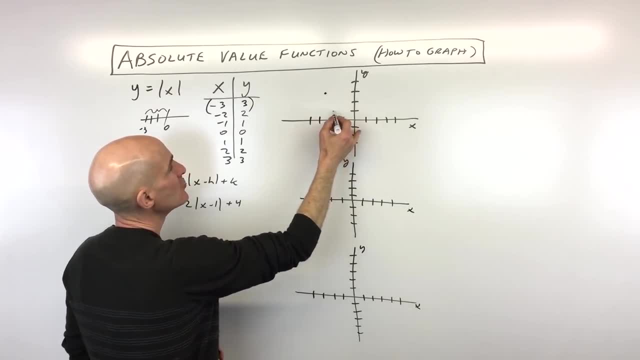 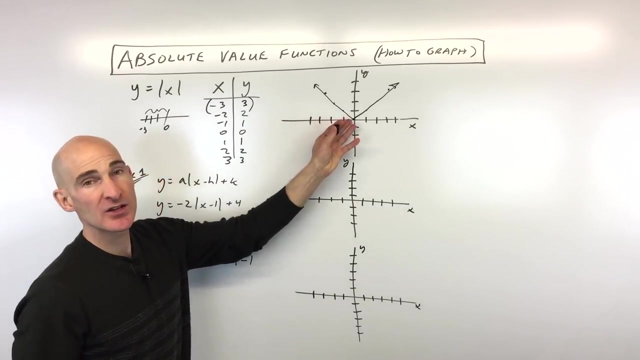 got left, three up three right, Left, two up two, left, one up one, zero zero one. one, two, two, three, three. And what you'll notice when you graph these absolute value graphs, it has that real sharp V shape, that real sharp corner to it. So that's our basic. 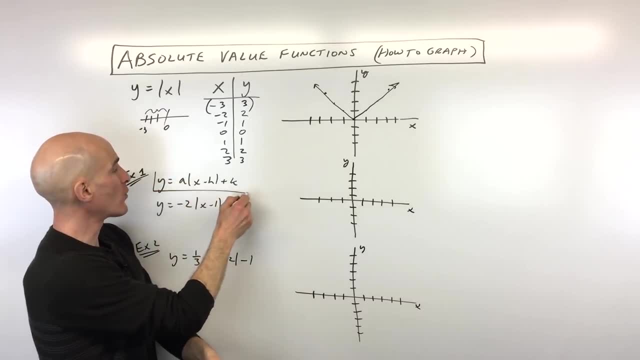 graph. But now let's say we want to do more challenging ones. Say, for example, ones that are in this form: here, Y equals a absolute value of x minus h plus k. So how does this work? Well, the h, okay. 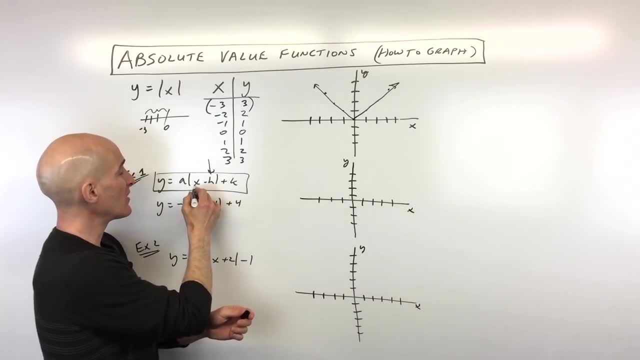 is what shifts the graph left and right. Okay, so this number that's grouped with the x, it's easy to remember. It shifts it in the x-axis direction left and right. But this one has the opposite effect on the graph. So that means if it's x minus two, it would 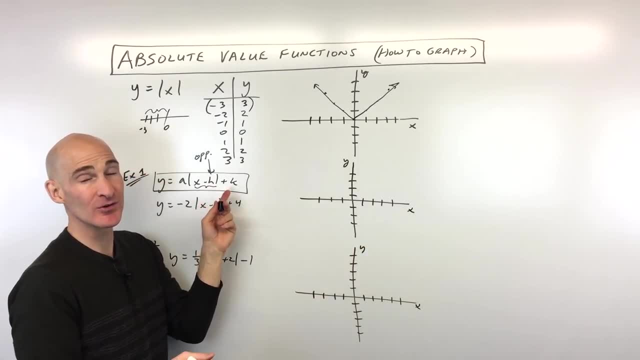 actually go positive two, so to the right. If it was x plus two, it would actually go negative two, so to the left, two. But this k value actually has the same effect on the graph, meaning if it's positive you're going to shift it up And if it's negative you're. 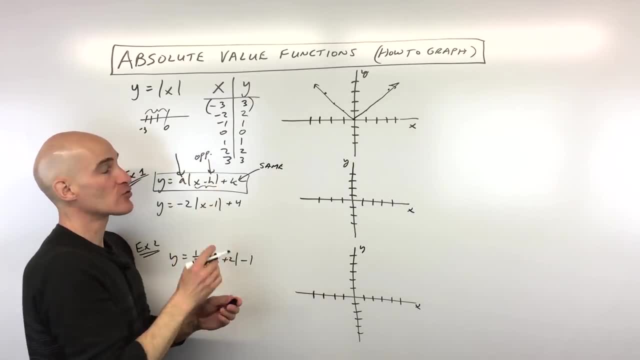 going to shift it down. Okay, then, what the a value does is it stretches the graph or compresses the graph, Okay, and if it's negative, what it'll do is it'll reflect the graph over the x-axis. If a is greater than one, it's a vertical stretch. If it's between zero and 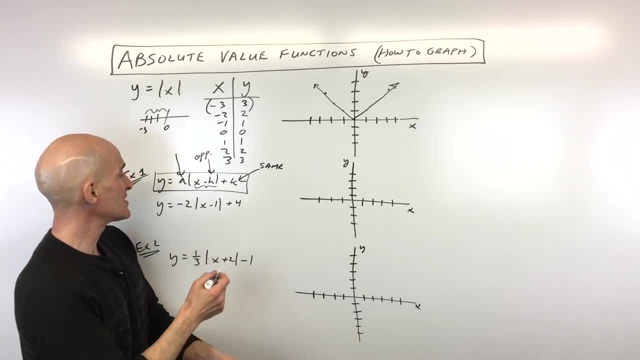 one like a half. it's a vertical shrink. Let's take a look at some examples so you can see how this works. So say, for example, this one here: y equals negative two. absolute value of x minus one plus four. Okay, what I like to do is I like to do the translation. 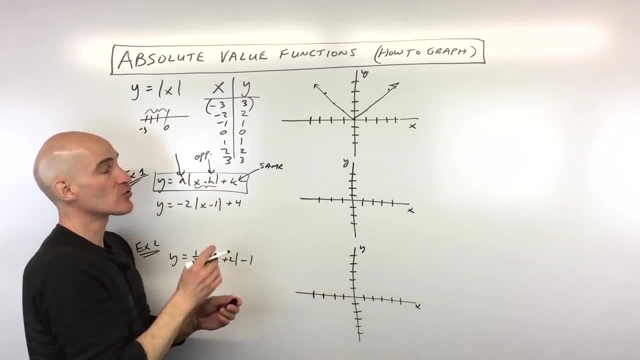 going to shift it down. Okay, then, what the a value does is it stretches the graph or compresses the graph, Okay, and if it's negative, what it'll do is it'll reflect the graph over the x-axis. If a is greater than one, it's a vertical stretch. If it's between zero and 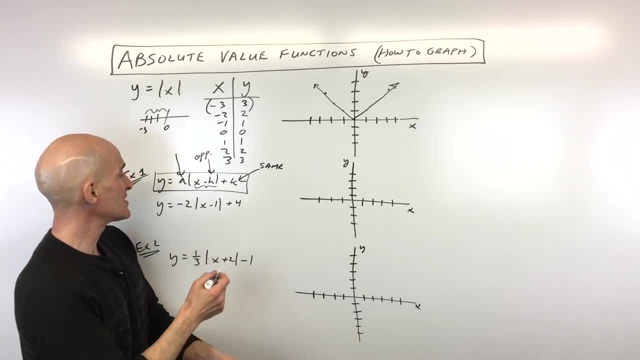 one like a half. it's a vertical shrink. Let's take a look at some examples so you can see how this works. So say, for example, this one here: y equals negative two. absolute value of x minus one plus four. Okay, what I like to do is I like to do the translation. 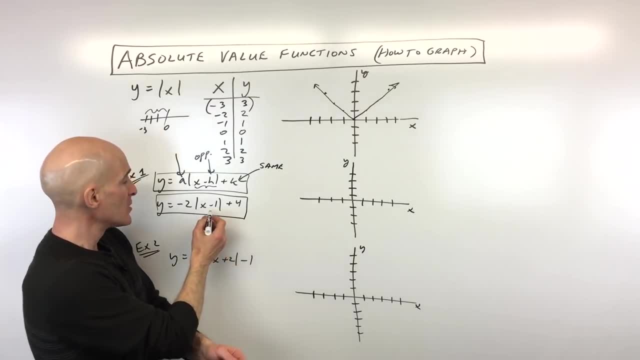 So I'm going to go to the next one. I'm going to go to the next one, I'm going to go to the next one. I like to do the translation or the shift first. So what does this minus one right here do to the graph? Okay, well, if you said right one, you're right, And then